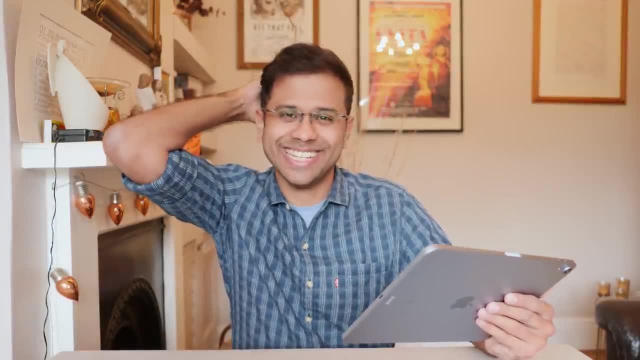 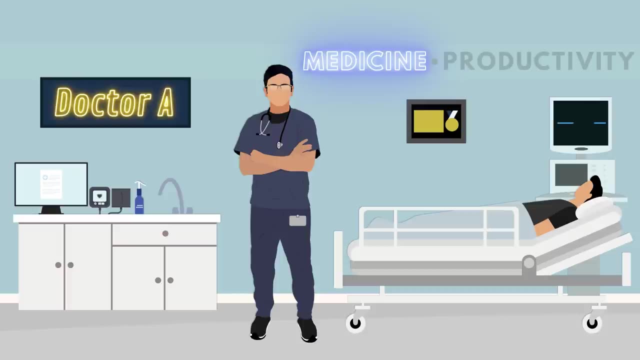 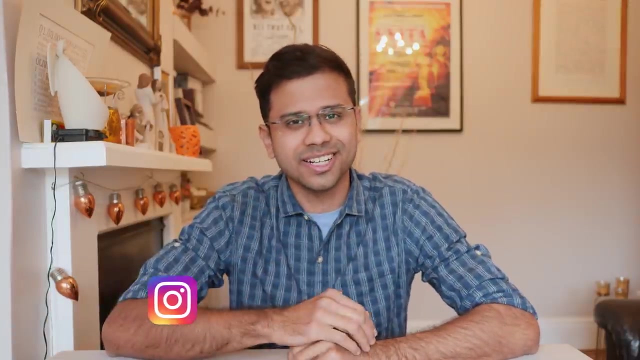 $9000?. Eyyy What? Hey there, lovely person watching YouTube. If you are new here, hi, my name is Ajay. I am a doctor from India. If you are already subscribed, welcome back. I love you to the stars and back. 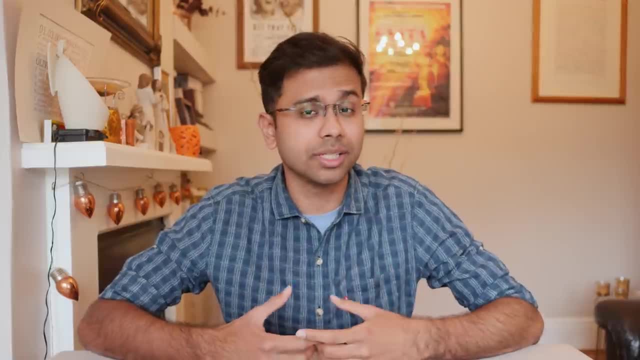 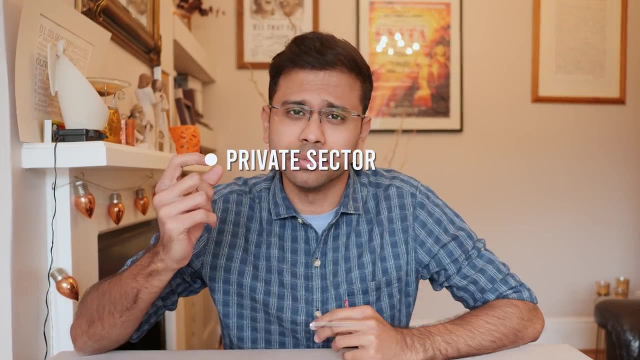 So healthcare in India, where I am from, is of two types. It is either given by the government, which is cheap and very affordable, or it is in the private sector, which is not very affordable. But if there is one country in the world that is very. 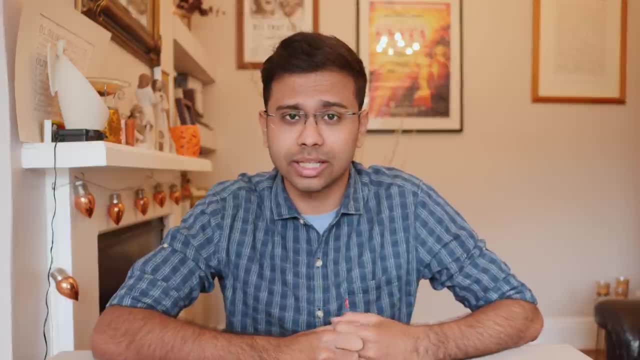 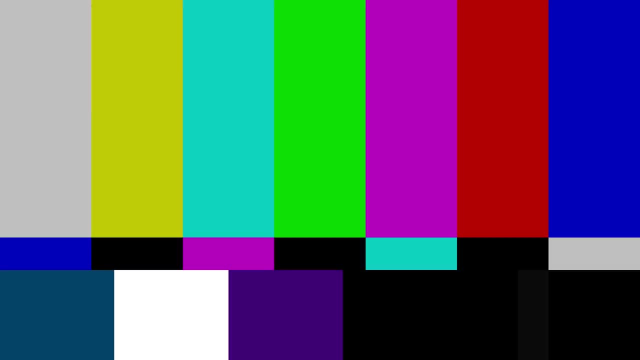 notorious for being very unaffordable when it comes to healthcare- like: if you don't have insurance, you are basically f**ked- is the United States of America. So today we will be playing an interesting game of guessing American medical bills. Now these are: 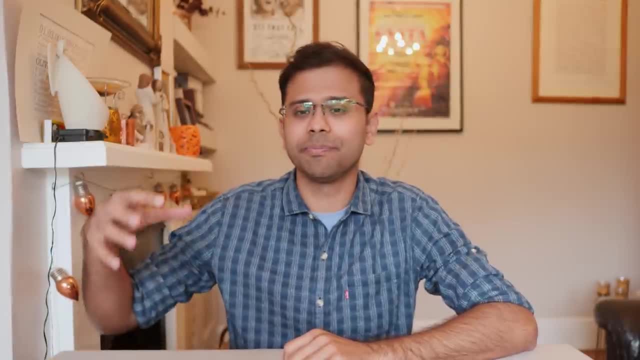 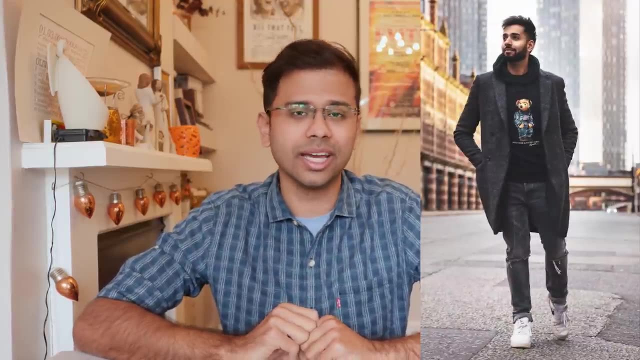 real medical bills from real American hospitals. These were made for us by someone- and I will be doing that with my good friend, Dr Kiran Mojaria, who is a GP trainee here in the UK, who went to medical school in the UK, who has been working in the NHS. 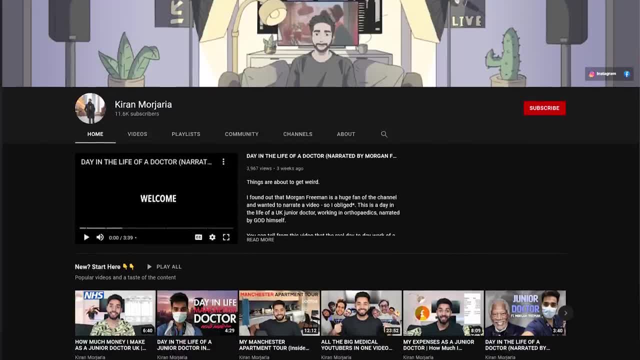 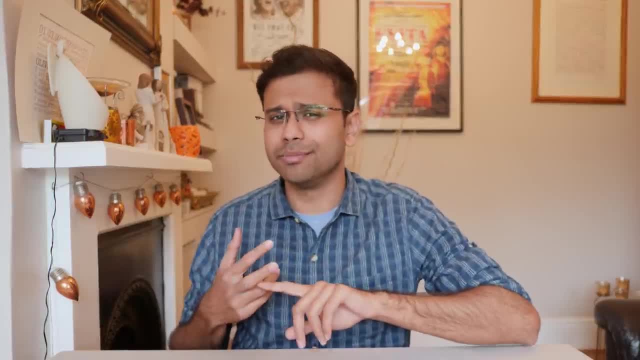 for over 3 years now. He also has an amazing channel on YouTube, so make sure you guys check it out after watching this video. So basically, the rules of the games are this. So I think there are around 4 to 5 bills real. 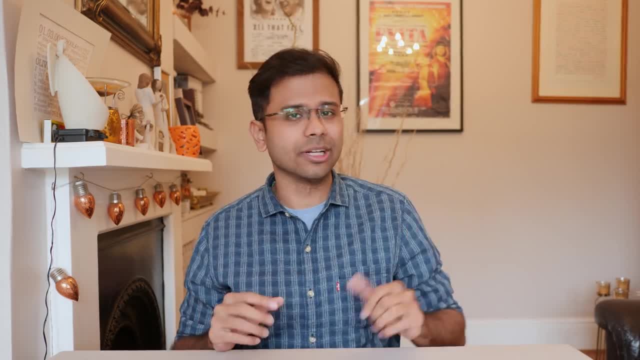 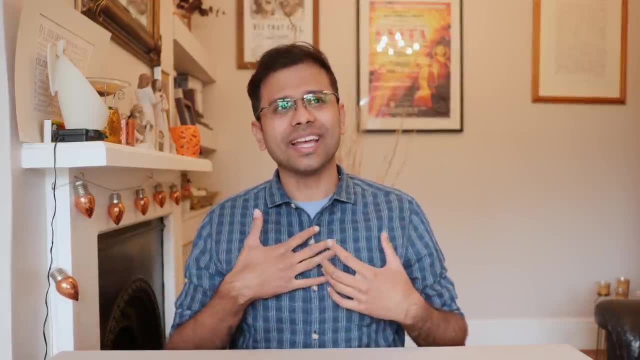 American bills, and both me and Kiran we are going to take a look at it and we are going to try to guess based on what we think it would cost. I think mine is going to be a bit different because I have worked in the private sector in India, so 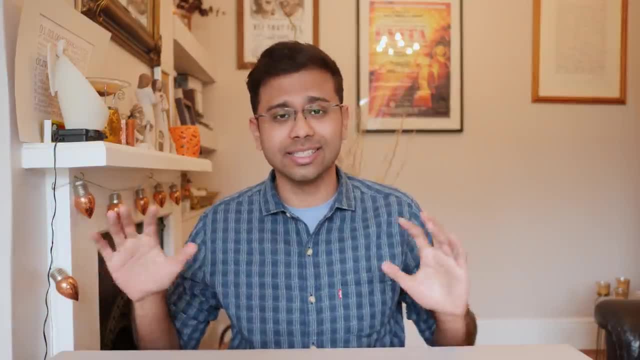 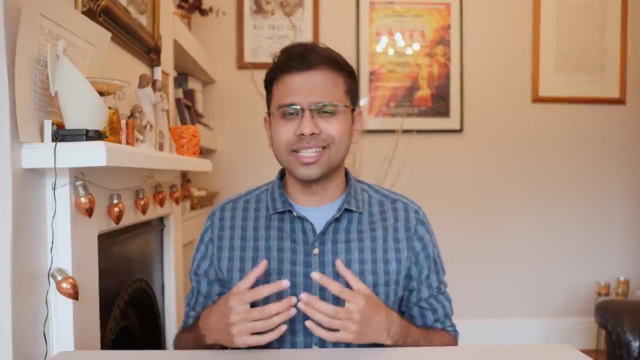 it's still a bit expensive, You know, at least by Indian standards it's expensive. Kiran has only worked in the NHS. Basically, in the NHS most of the things are free, So I think it's going to be interesting to see how much we 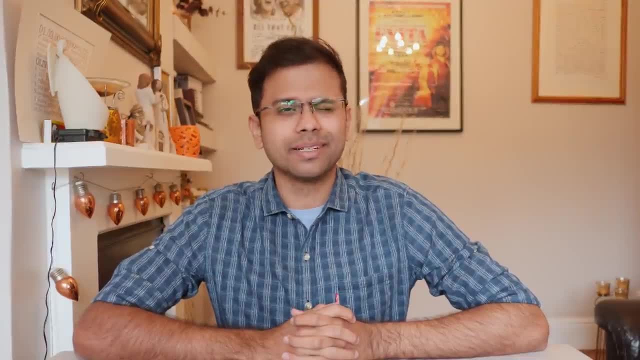 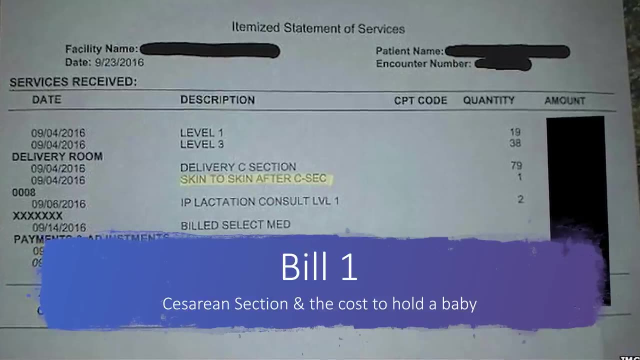 both guess these prices, as I know it's going to be bad. but how bad are these bills? Let's see. So bill number 1 is caesarean section and the cost to hold the baby In India in a. 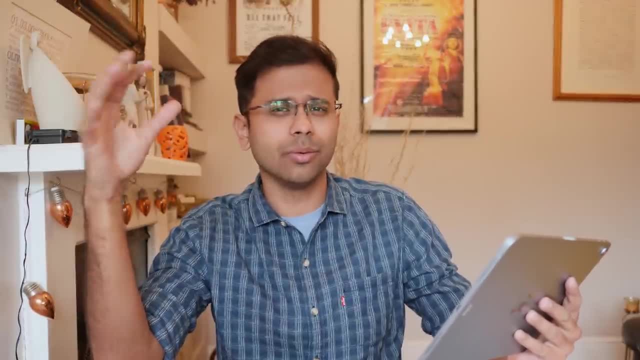 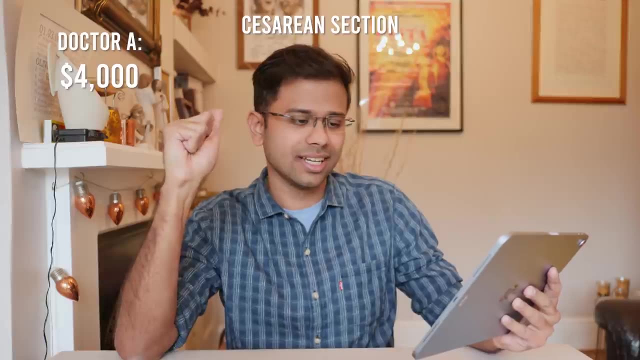 very good hospital. it would be around 4 lakh rupees. if you want like the best hospital with like VIP suite and all that, I'm thinking it's going to be around 4,000 dollars, But I think it's going to be more than that, I think. 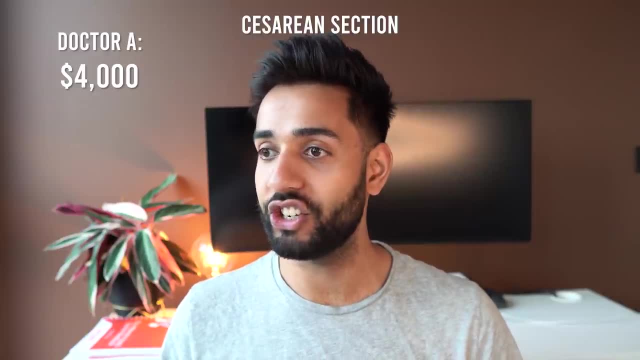 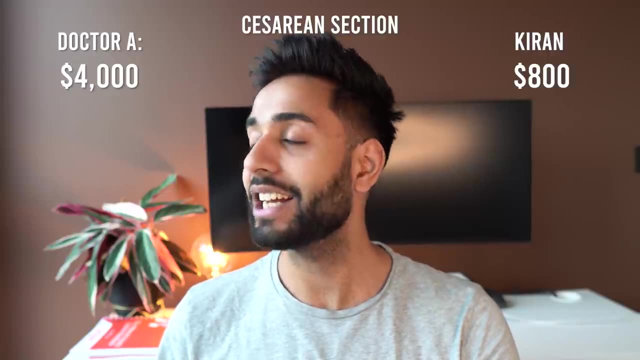 you know, it's a surgery. there's an anaesthetist, there's going to be a surgeon, there's the operating theatre. I think it's going to be expensive. Let's go for 800 dollars. It's 3,000. 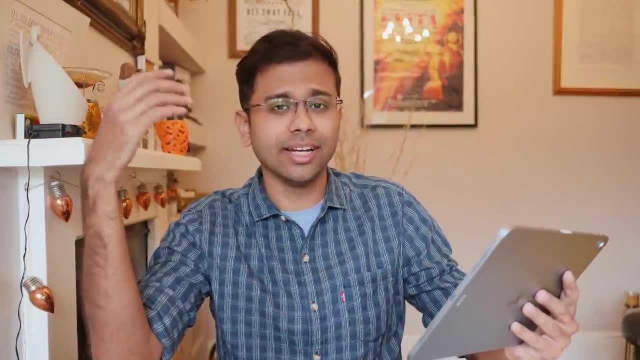 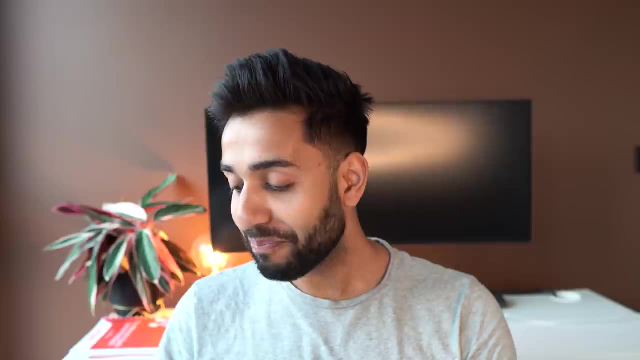 dollars, which is not too bad if you ask me Like. we have Indian hospitals which charge more than this, so I'm not very surprised by this. This is actually pretty decent if you ask me 3. 3,100 dollars. 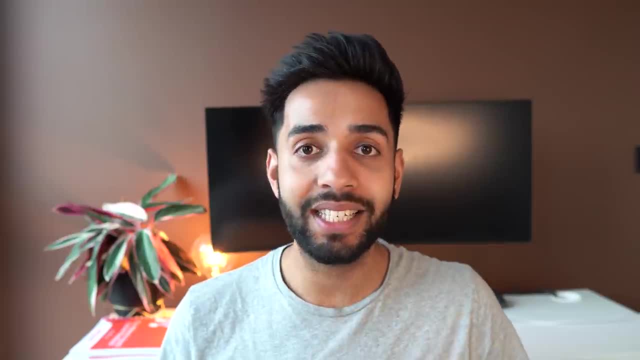 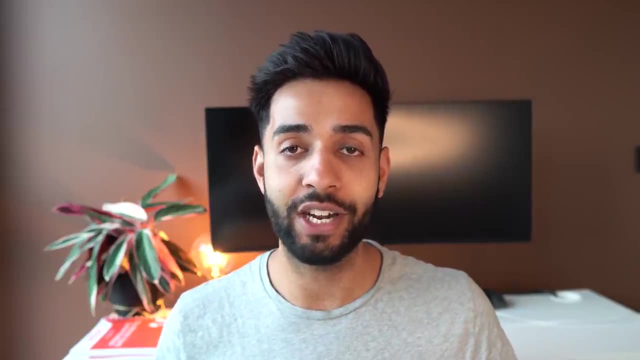 to have a C-section, And bear in mind that some C-sections aren't even planned, so this may have been an emergency C-section. So imagine going for a normal delivery and then it being converted to a C-section and then being whacked. 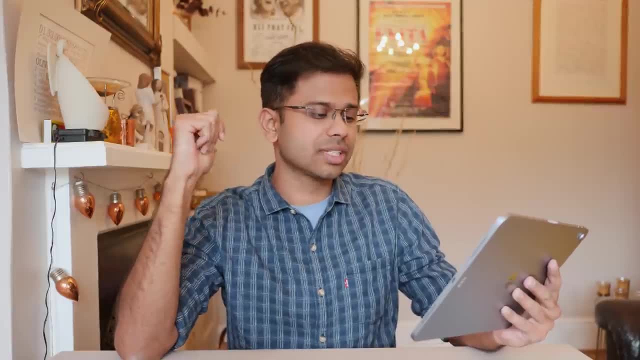 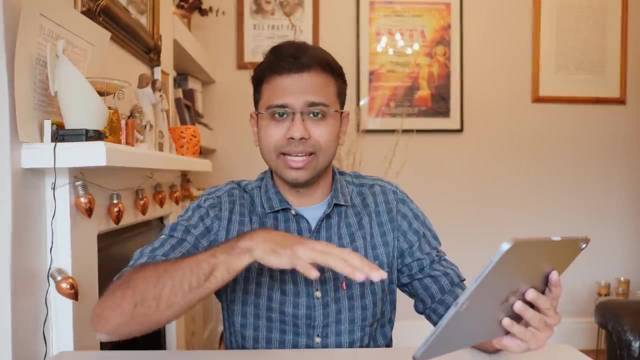 with a bill of 3,000 dollars. So then, skin to skin after C-section. So, basically, what skin to skin means is that when the baby is delivered, we put the baby on the mother's belly so that there could be some one. 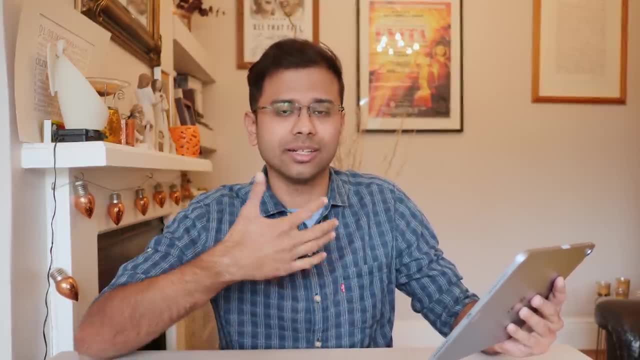 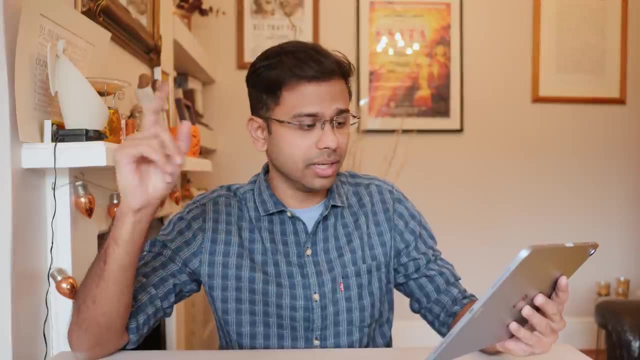 bonding and second heat exchange between the mother and to the baby to keep the baby warm, basically. So there's a lot of evidence saying that this is a very ideal thing to do, but apparently they charge them for that. I have no idea why. So 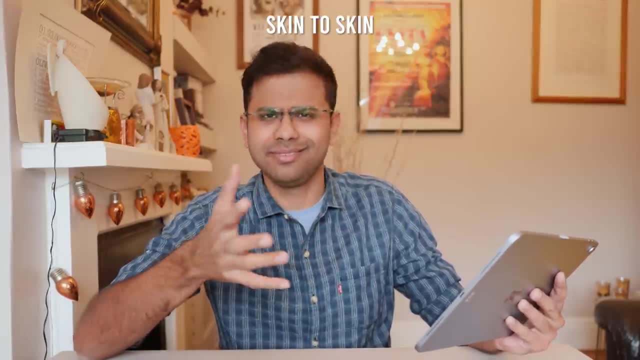 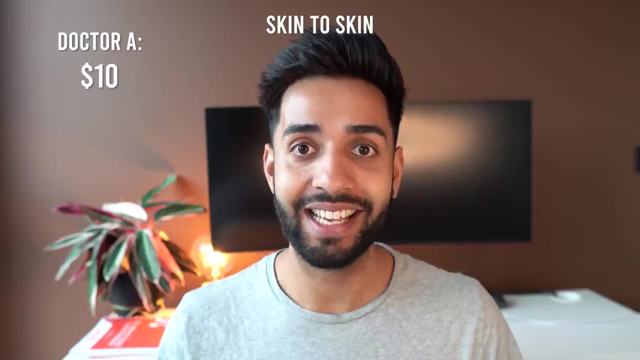 I don't know how much they charge. I'm guessing around 10 dollars, 20 dollars, because you shouldn't be charging for this. but let's see. First of all, I'm surprised that they're charging for this, but I'm gonna. 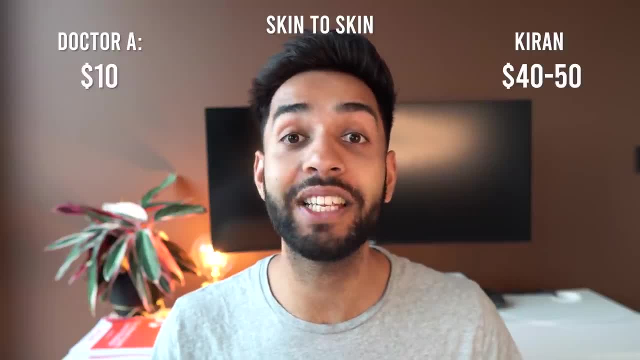 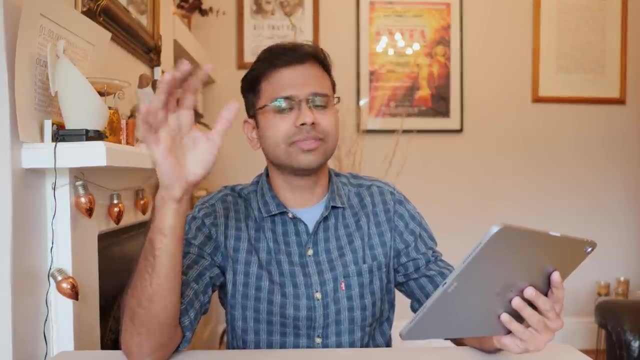 guess it's gonna be very cheap. Let's say, 40, 50 dollars, 39 dollars, 35 cents- I don't know why they're even charging for that. Okay, not very expensive. 40 dollars, okay, Well, I think. 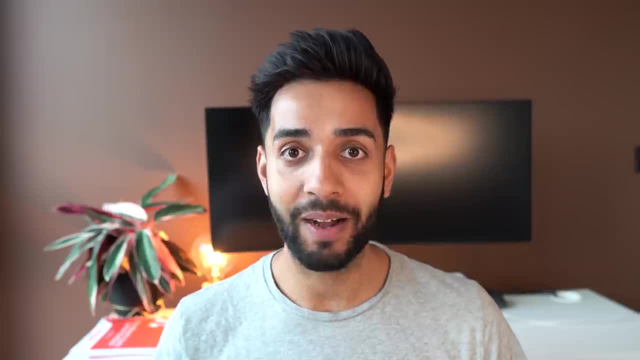 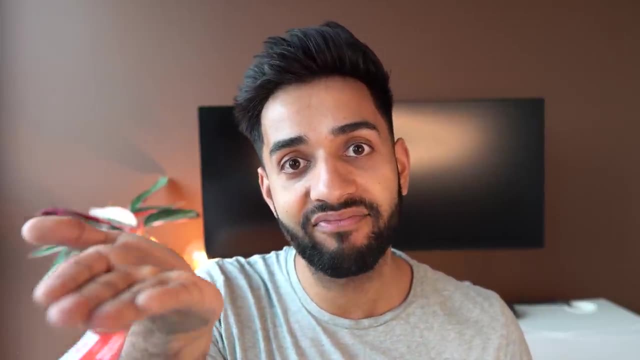 it's pretty astonishing that they've charged for that anyway, but at least 40 dollars is kind of reasonable Here. hold your baby, and that'll be 40 dollars, please. Next one: Inpatient lactation consultation, level one, because this is. 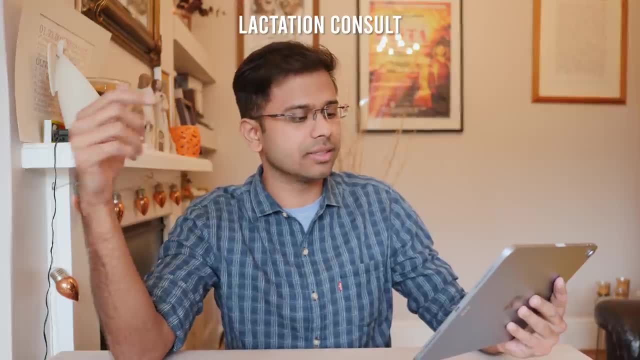 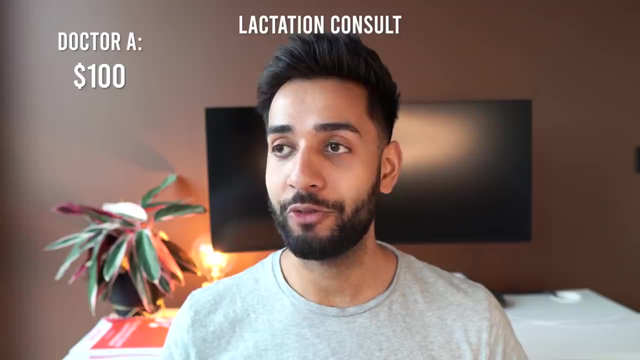 going to be like advanced nurse practitioner or like a doctor giving the consultation on how, to you know, feed, breastfeed the baby. I think this is gonna be around 100 dollars For a consultation like this, which is probably just some advice. 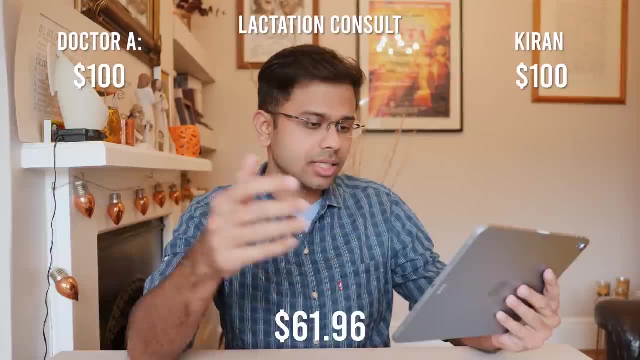 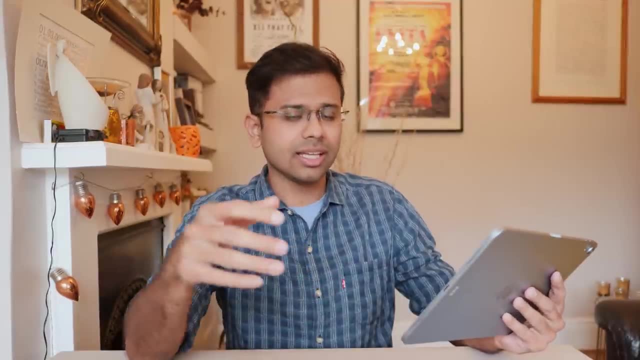 let's assume they've paid 100 dollars, 61 dollars, You know, this is actually quite affordable by American standards. if you ask me, I'm being very honest about it because I think even Indian hospitals- a lot of them- charge this much. So I'm not. very surprised. Let's compare this to the cost in the UK. So the C-section would have been free, skin to skin would have been free and the lactation consult would have been free as well. Next up, this patient presented with stomach pain. 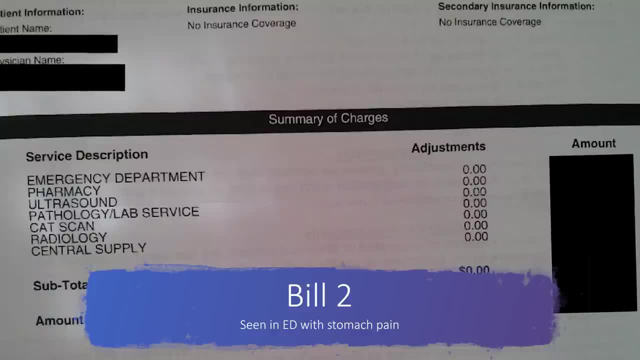 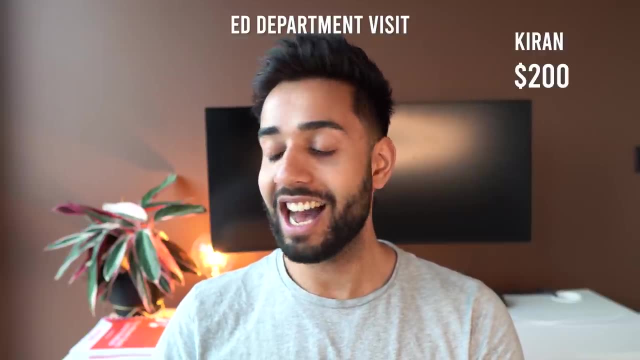 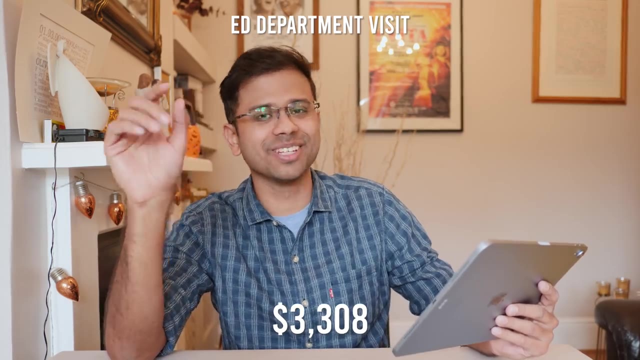 to the ED was given morphine, a PPI, a CT scan and released six hours later. So the cost for the emergency department visit, let's guess a couple hundred dollars, Three thousand dollars, Whoa Three thousand dollars for just going into the emergency department. 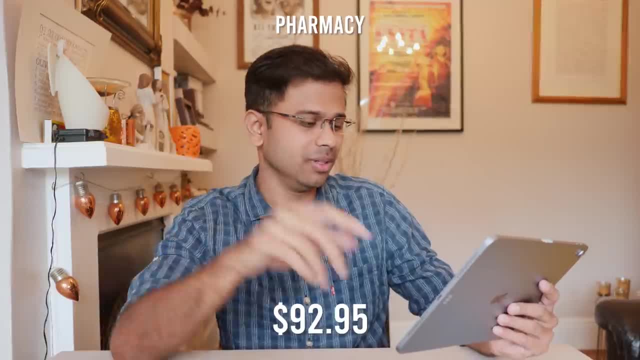 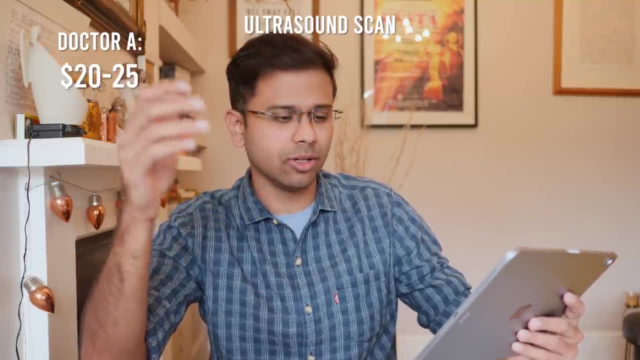 Pharmacy fees are 92 dollars. That's okay, affordable. So ultrasound scan in India it would be around 1500 rupees. So that's what like 20-25 dollars The ultrasound scan. bear in mind, that's just a. 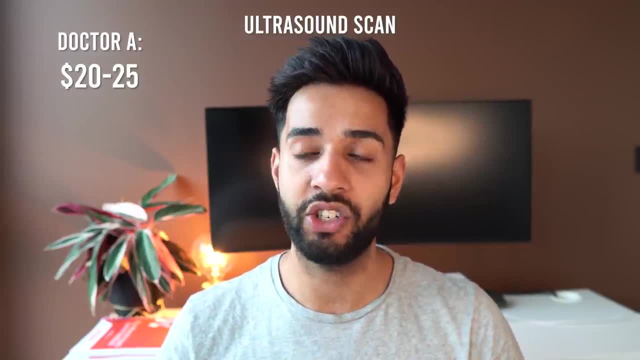 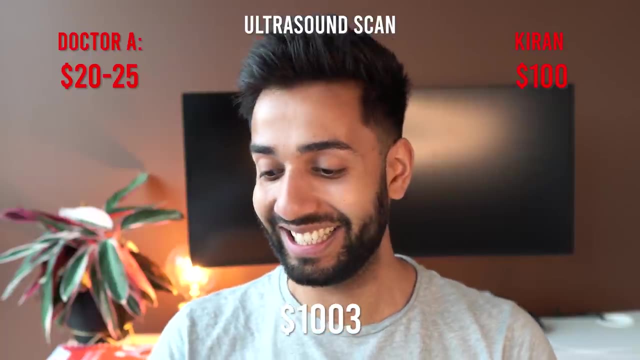 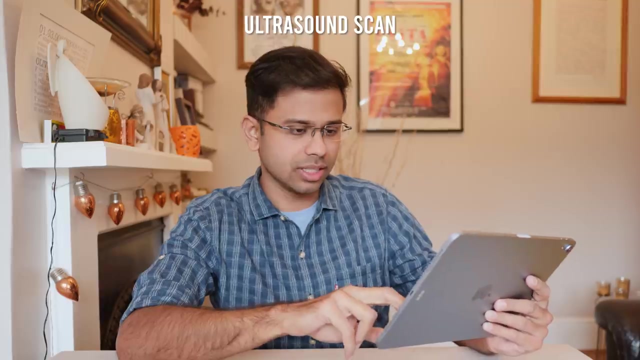 jelly scan. The actual cost of that is just the cost of the person doing the scan. So let's go for a hundred dollars. A thousand dollars. To have an ultrasound scan cost one thousand dollars. That's insane. We give them out like sweets here. So let's see how much. 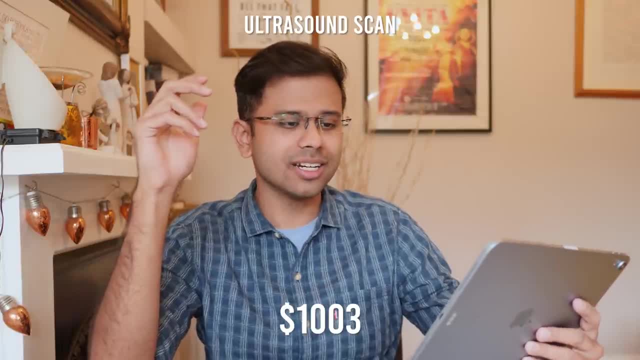 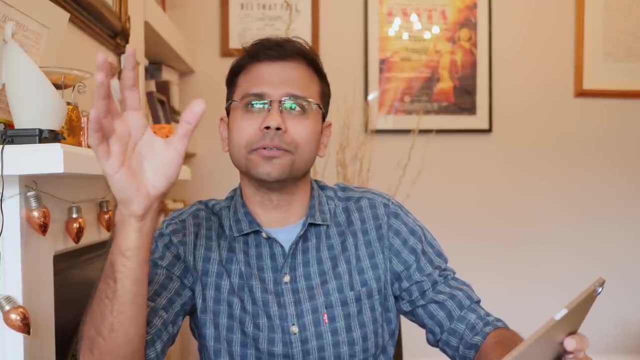 it is, It's gonna be expensive. Thousand dollars for an ultrasound, Are they crazy? A thousand dollars is like 70 thousand rupees- Like you could literally get like some 30-40 ultrasounds in India for that cost. This is very expensive. 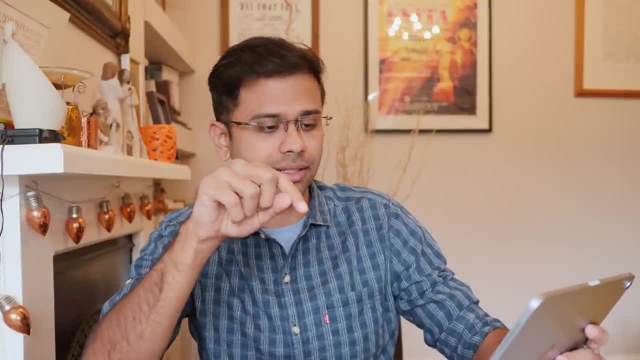 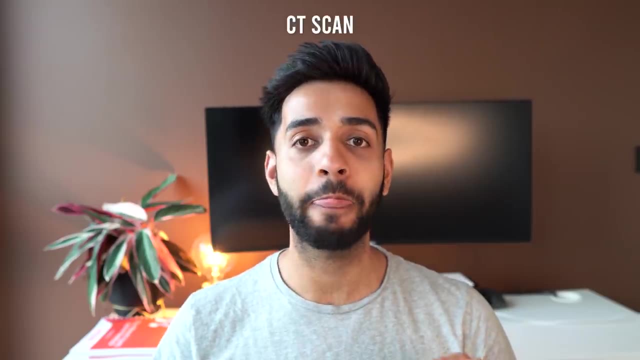 Maybe this is because it involves a radiologist, but even then they shouldn't be charging so much. A thousand dollars for an ultrasound is crazy For the CT scan. the CT scan surely has to be more expensive than the ultrasound scan, Which was a thousand dollars. So I'm gonna say a thousand five hundred dollars- I just had to read it twice- Six thousand eight hundred dollars for a CT scan. Six thousand eight hundred and sixty seven dollars. Six thousand dollars for a CAT scan. I think in India it would cost like a maximum. 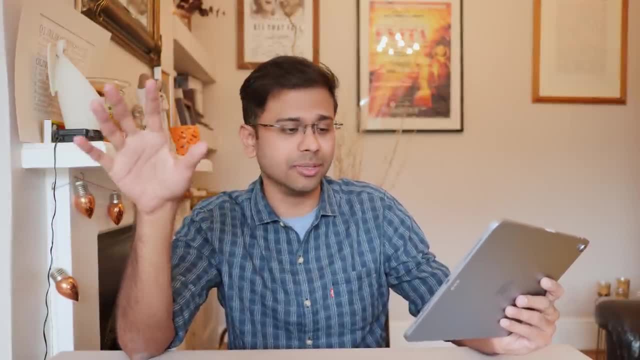 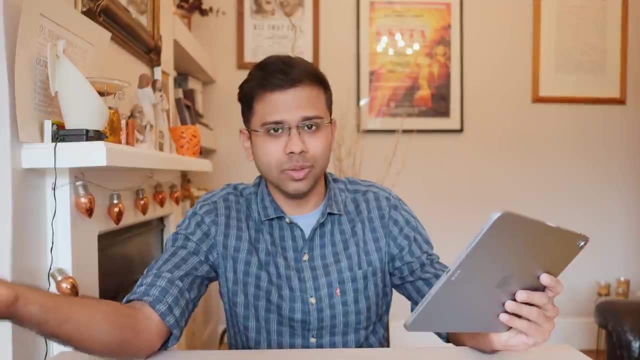 of two hundred dollars, even at a very good facility with very good CT machines. And I think in the UK, here in the UK it's free because it's done only if you need to do it and the trust pays for it. Basically, the government, the NHS, pays for it. So here it's six thousand eight hundred dollars. I just can't get my head around the fact that this CT scan was six thousand eight hundred dollars. I ordered like five of them today for free. Radiology is four hundred forty five dollars. Maybe a doctor consult? 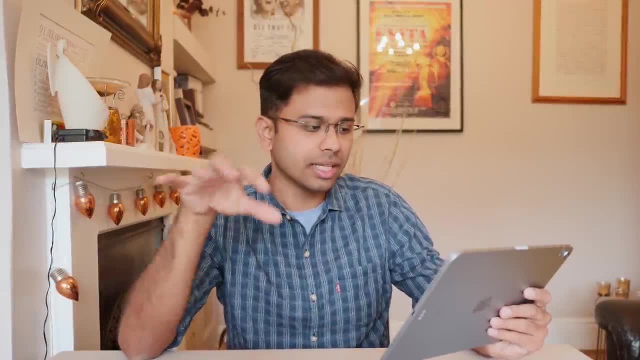 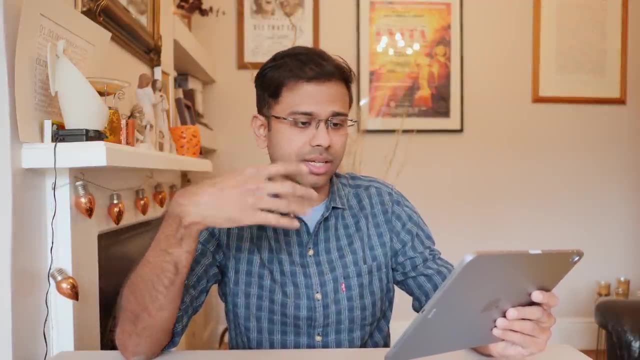 But four hundred forty five dollars for a consult is quite a lot, But I think this also. radiology also includes an x-ray, chest x-ray, abdominal x-ray and other x-rays, Because this guy was in a trauma. So if that was the case, 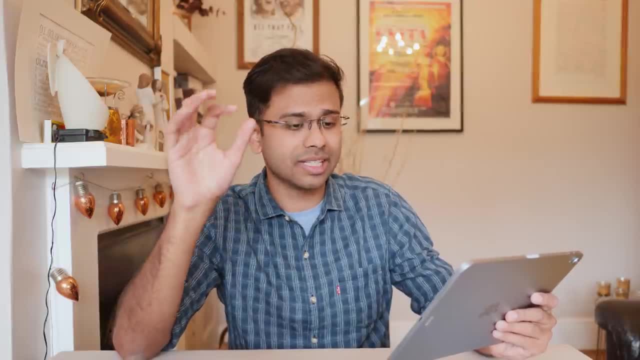 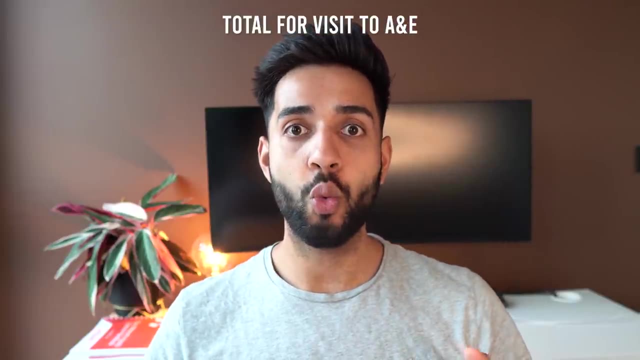 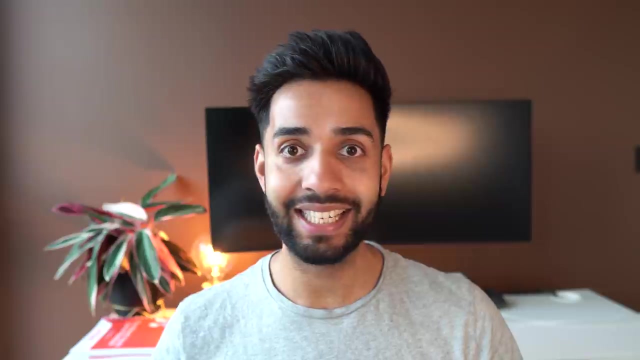 four forty five is still not justified, but it's okay. But if it's just the doctor's opinion, four forty five is crazy money. The total for this visit to A&E was twelve and a half thousand dollars. Imagine having stomach pain going to ED, having these scans. 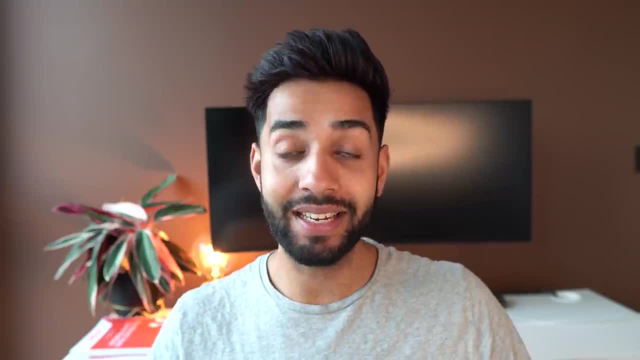 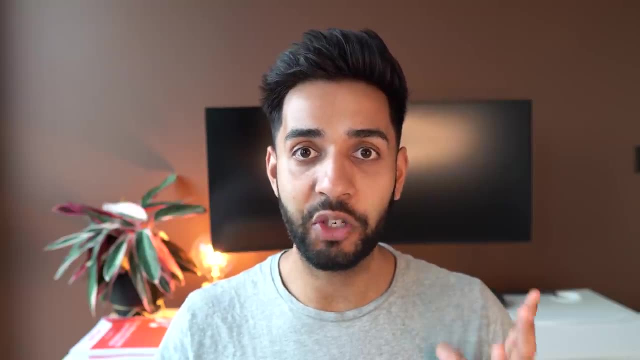 getting some morphine, getting a PPI and being discharged with them saying actually it's just gastritis which doesn't need anything further doing, and then getting a bill for twelve and a half thousand dollars If you don't have insurance and you have a bill like 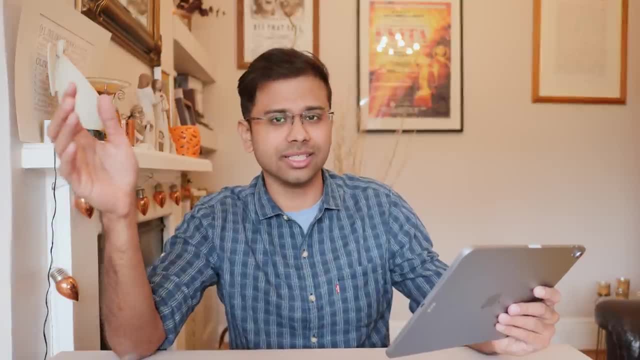 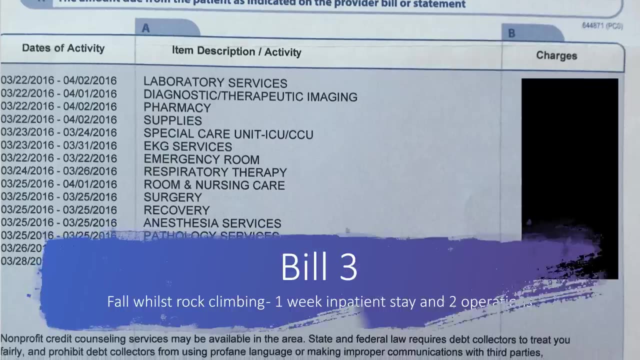 this. that's going to take away like a quarter of your year's salary for just this one day, like some six hour visit to the emergency department. And that's crazy. Bill number three: This patient fell while rock climbing and broke his neck back. 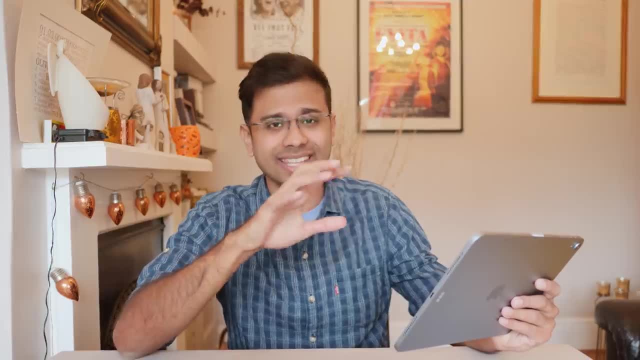 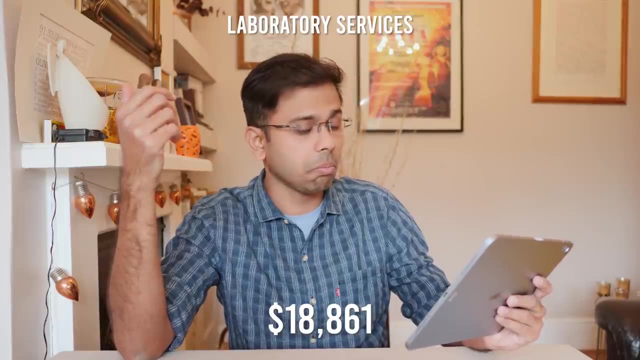 and ankle, Had two operations and a week in a hospital. This guy- I hope he has insurance, So this is from 2016,, so fairly recent. Laboratory services: eighteen thousand Quite a lot. Let's see Diagnostic therapeutic imaging. This guy has had a lot. 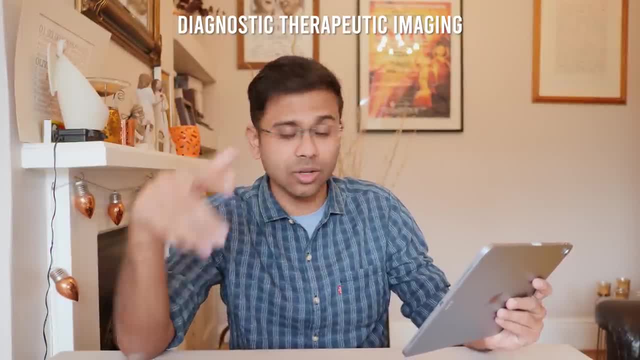 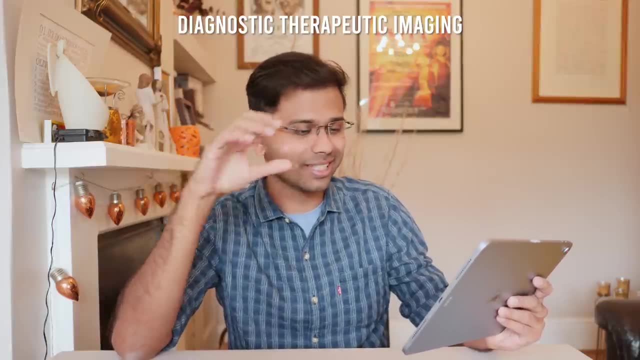 of fractures. So I think there will be a lot of x-rays and a lot of CT scans, or CAT scans like the Americans call it. involved A lot of ultrasounds involved. So if the labs took eighteen thousand, I'm just taking a wild guess that. 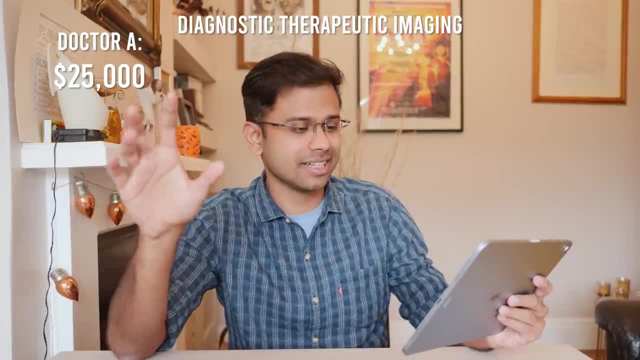 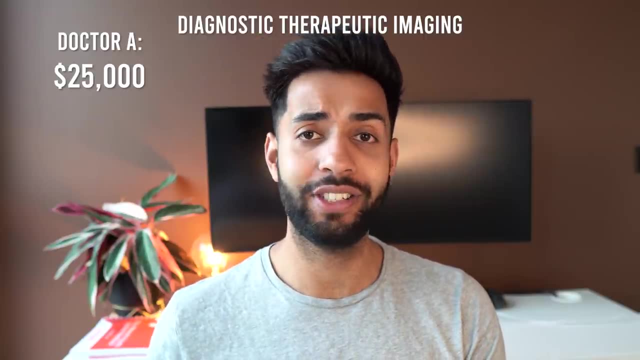 imaging would have taken like some twenty five thousand dollars at least, But let's see The imaging. so I don't know how much imaging this patient had. We know a CT scan is costing six thousand dollars, So I'm going to go ten thousand dollars. 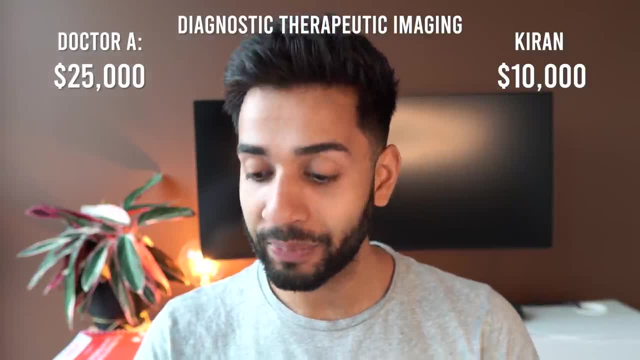 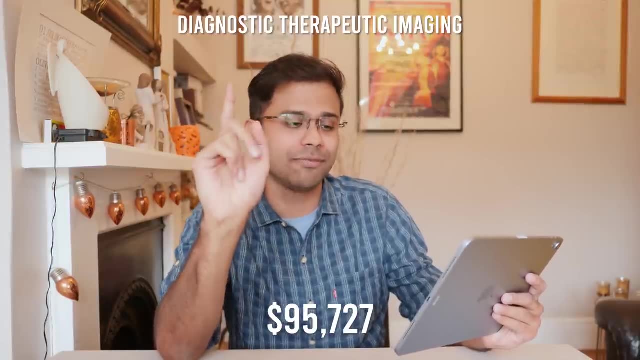 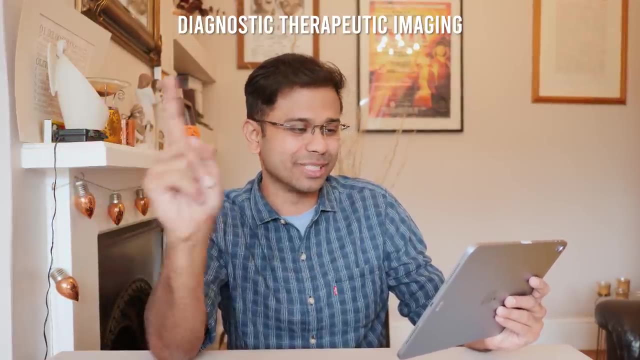 It's actually. it's actually funny how expensive this is. Ninety five thousand. So just for imaging, they've charged him ninety five thousand dollars. That's like more than a resident's salary in the US. Oh god, But just one. 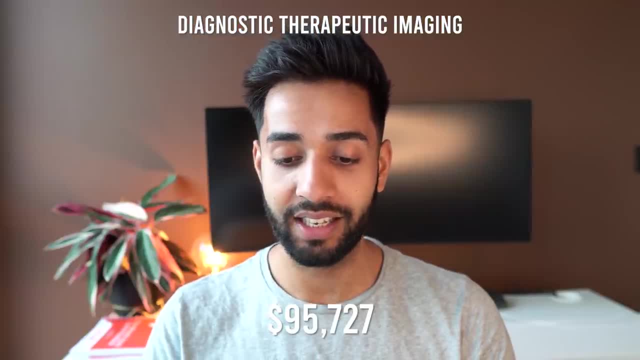 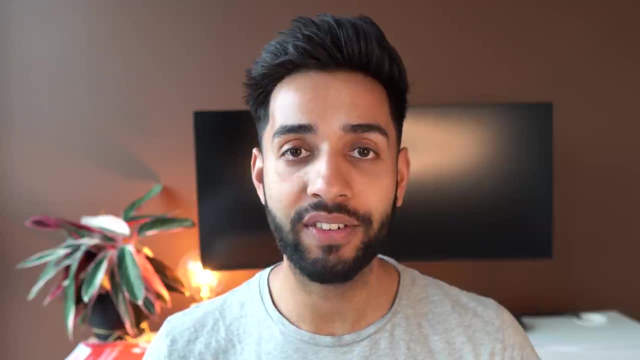 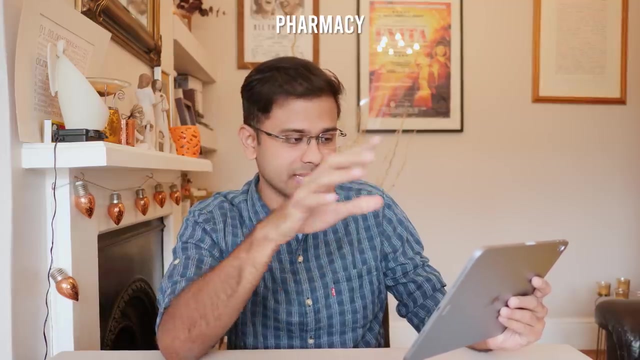 week. Ninety five thousand dollars for imaging. Did they give this man the MRI machine? I would be disappointed if I went to hospital, paid ninety five thousand dollars and didn't get the MRI machine to come home with. This is crazy. Next pharmacy: 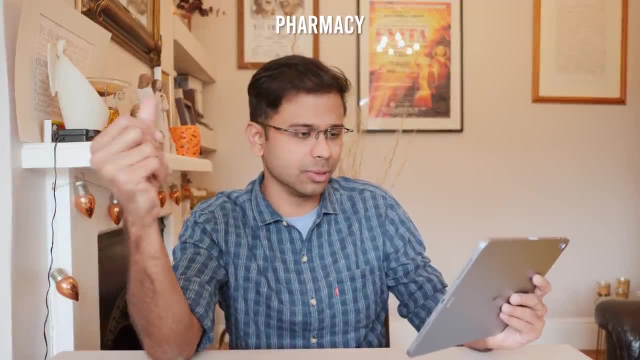 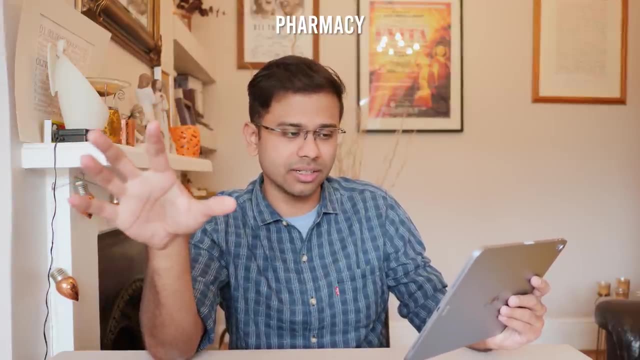 Basically all the drugs or the medicines that they would have used. I'm guessing, because he was in the hospital, he would have had multiple surgeries, So I'm guessing, around ten thousand dollars. But it's the US, so it's thirty three thousand dollars. It's just a little thirty three thousand dollars worth of medication for his one week's worth of inpatient stay. So ICU it was charged thirty thousand, which is okay, because ICU there's so much happening. You need to pay so many nurses, so many doctors and 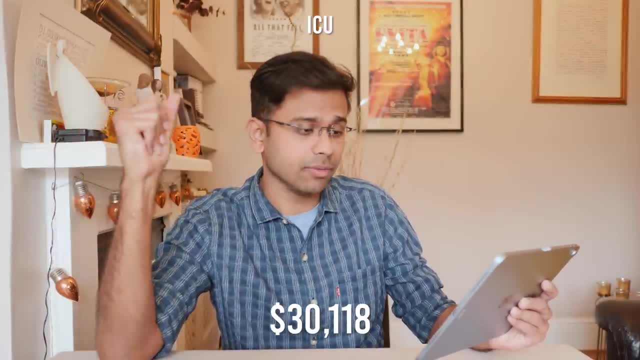 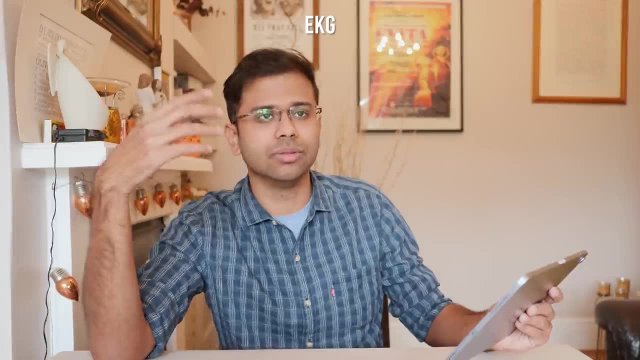 there's so many equipments, everything you have to pay for it. So thirty thousand, even though it's more by American standards, I think that's okay. But then EKG services, so electrocardiogram, ECG. I don't know why they call it. 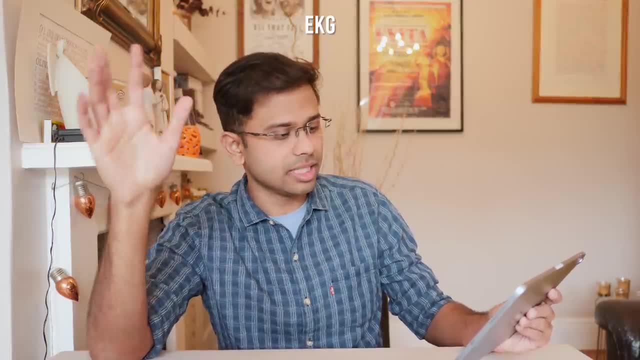 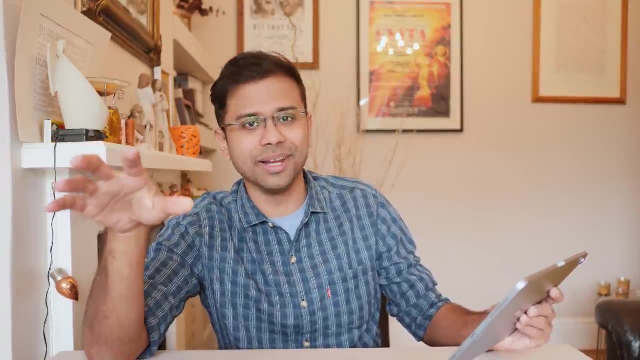 EKG- Electrocardiogram with a K. But basically EKG services is basically taking ECG's and because he was in the ICU, I think a lot of ECG's would have been done In India. it would be like some three hundred rupees. 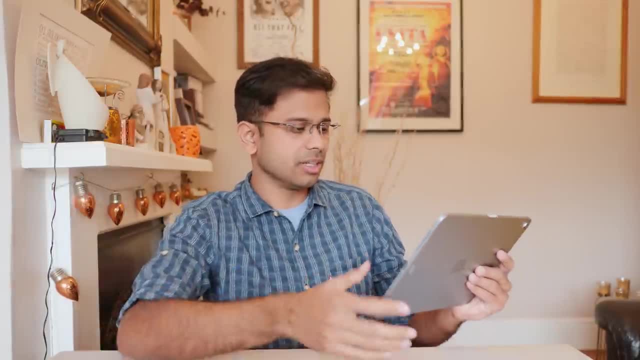 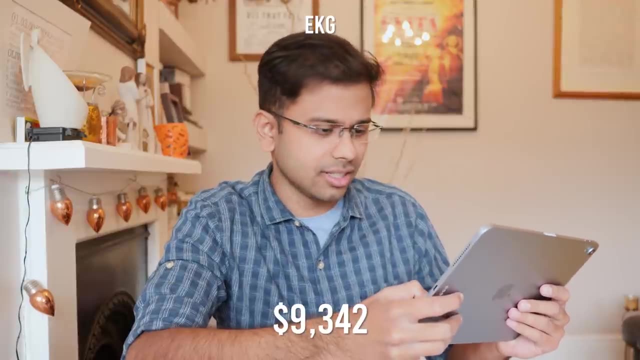 for an ECG. so it's what like five dollars or whatever. But in the US healthcare everything is expensive. So let's see how much they billed him for EKG. Nine thousand dollars, Like. how many ECG's did they take, Like how. 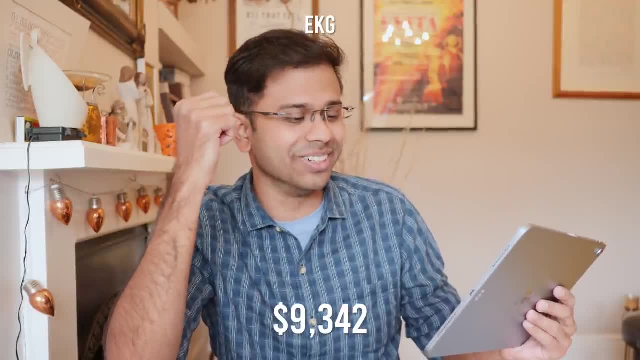 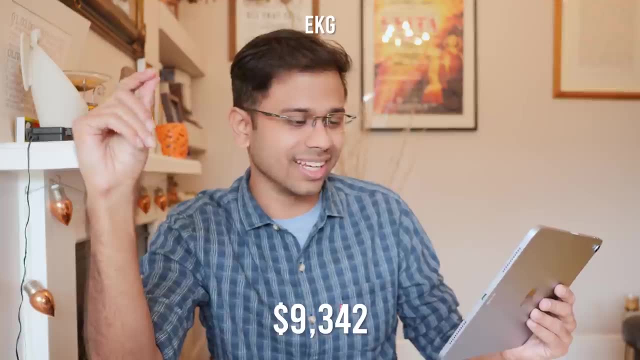 can someone take ECG's worth nine thousand dollars Like literally he was probably on like ECG like throughout his whole stay or something Like it just doesn't make sense to me. This is weird- EKG's in the UK we call ECG's and actually 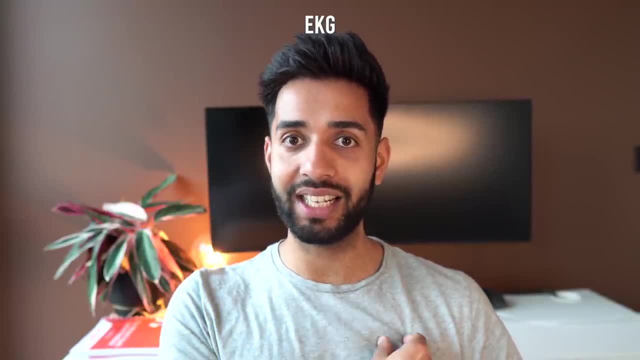 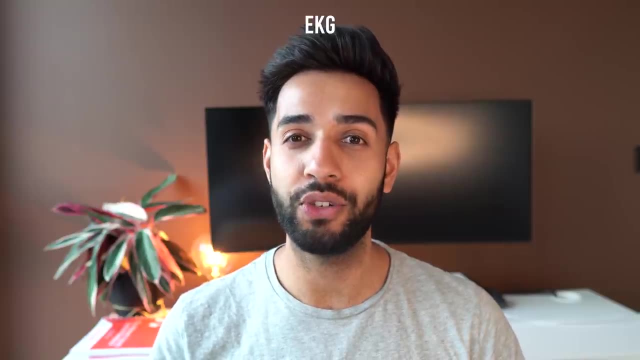 the cost of these shouldn't be much, because you just stick some stickers on and then do an ECG. So I'm gonna guess that this was a thousand dollars. A thousand dollars would be a lot for this, It's just a cheeky nine thousand dollars. 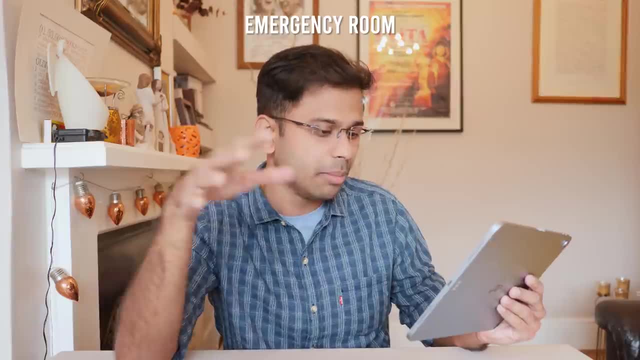 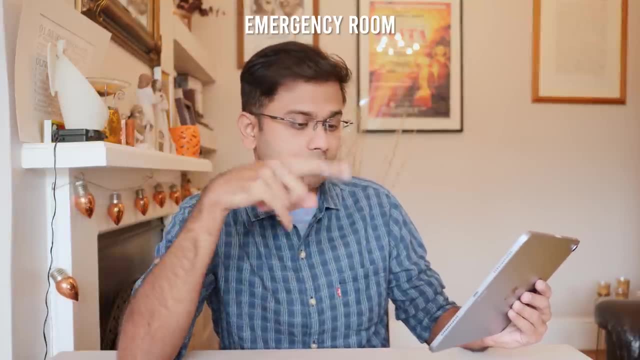 That's ridiculous. And then the emergency room. because he came into the emergency room, I think they would have charged him for the emergency room services, the doctors, the nurses and all that. So I think, based on the previous bill, I would guess around three thousand five thousand. 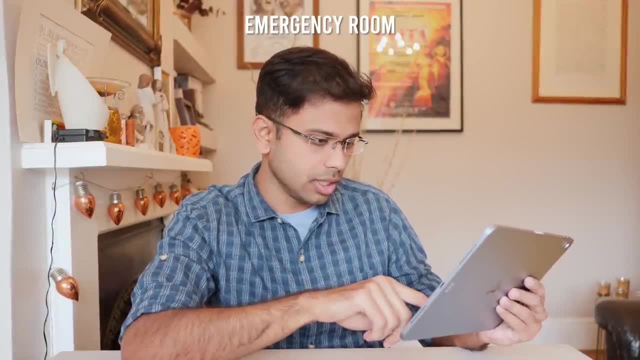 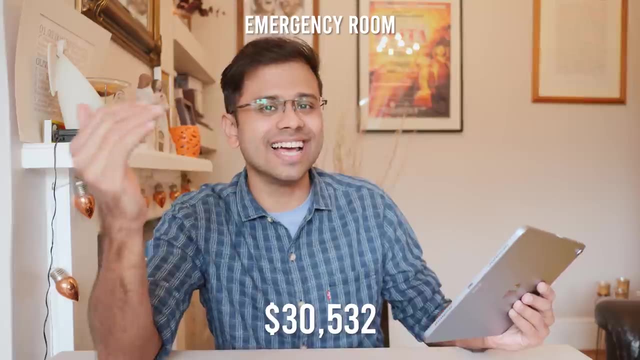 dollars. Let's see Emergency room. What Thirty thousand Dude? what are they gonna do for thirty thousand dollars? It's like half of a resident's yearly salary in the US. What are they gonna do with thirty thousand dollars? Again, this is daylight robbery, if you ask me. 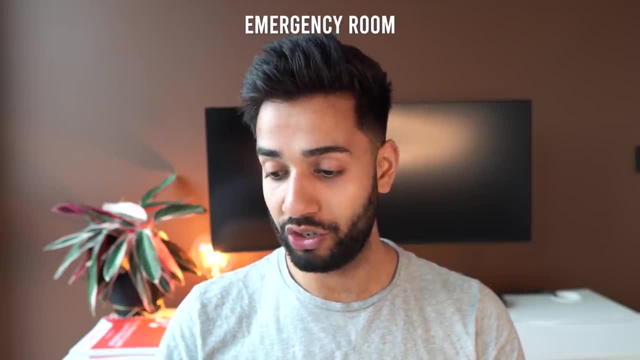 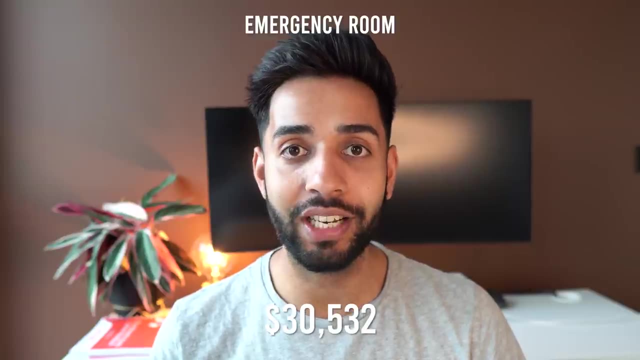 There's no other way to describe this. The emergency room was just another thirty thousand dollars. Imagine going to A&E and paying thirty thousand dollars. I actually can't even get my head around how much that is. I really hope this patient had insurance. 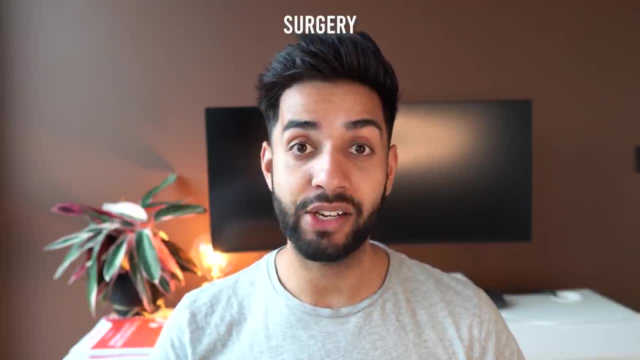 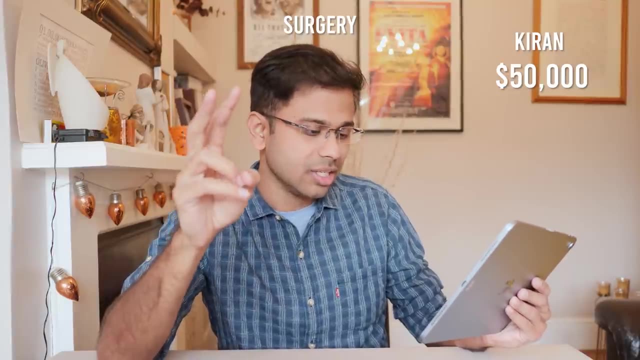 The surgery cost. If the scans are that much, the surgery has to be way more. So I'm gonna go fifty thousand dollars. Again, this guy was in surgery, Two surgeries, So that would have been a lot of money and, following the theme, I'm gonna guess a hundred. 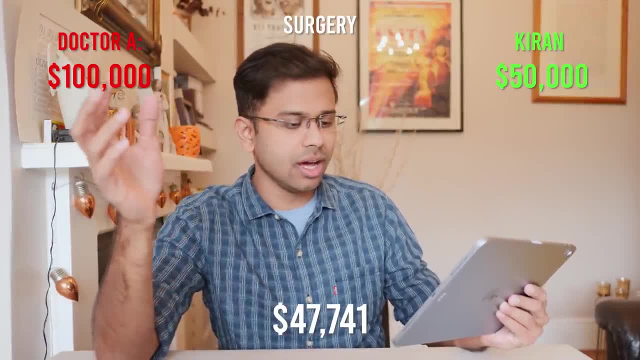 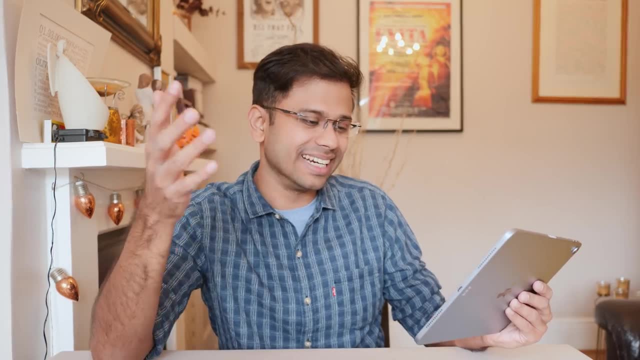 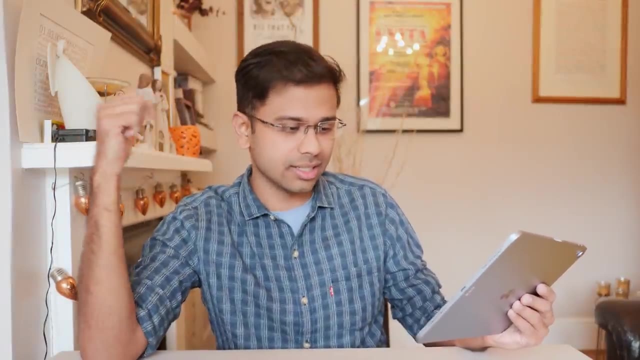 thousand dollars for the surgery. Forty-seven thousand dollars, Not too bad. comparing it to, you know like how much, like imaging and all took. It's weird, right? Like imaging is ninety five thousand dollars and surgery which involves so many doctors, specially trained doctors, so many nurses. anesthetists, everything is forty-seven thousand dollars. So I think they're, you know, ripping people off in the imaging and diagnostic services and they're cutting costs in surgery. So all in for that operation was fifty thousand dollars for the surgery and also. 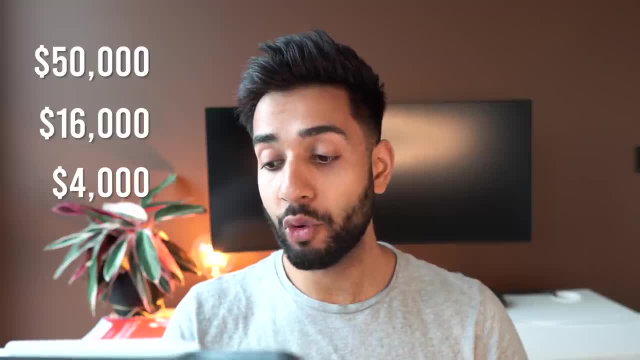 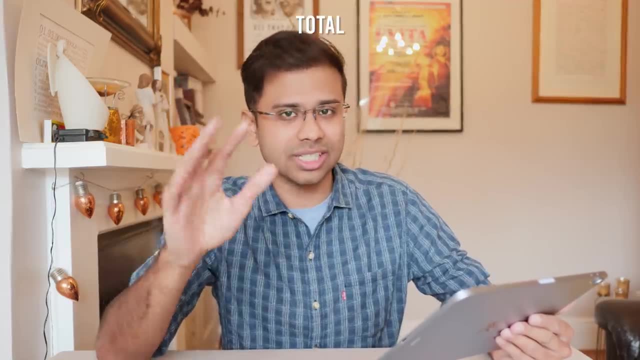 sixteen thousand dollars for the anaesthetist, Four thousand dollars for the recovery. So that operation itself cost seventy thousand dollars. So the total charges for this guy who broke his neck while rock climbing- I should have been more careful, but it is three hundred. 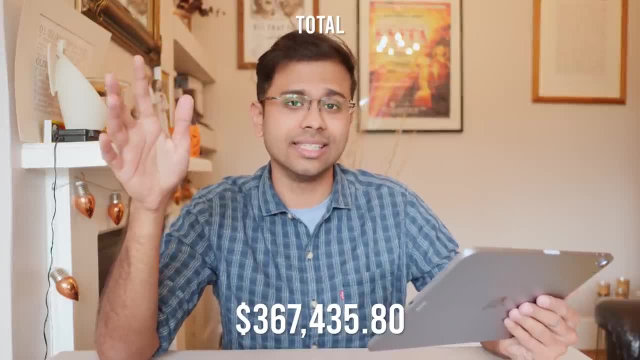 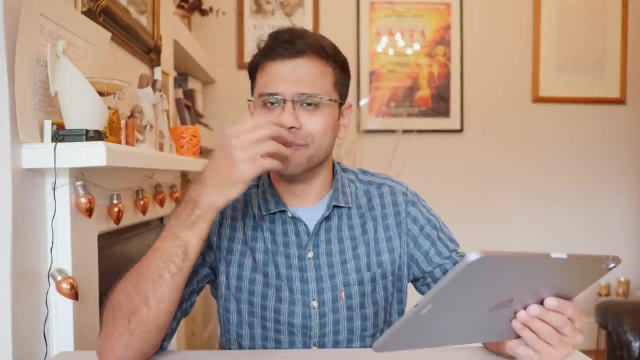 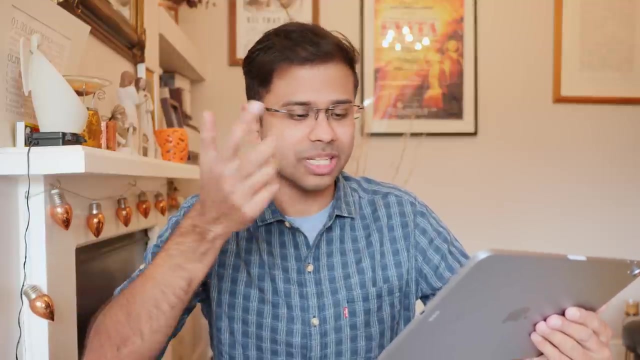 sixty-seven thousand four hundred and thirty-five dollars and eighty cents, and that's much more than most junior doctors net worth, Even a lot of mid-range doctors net worth in India and even in the UK. Doctors make a lot more in the US, but even then this is a ridiculous sum of money. for one accident. Three hundred sixty-seven thousand is like someone can literally retire with that kind of money, right? Can you imagine going to hospital, staying for a week and being hit with a bill of three hundred sixty-seven thousand dollars? That's going to take decades.